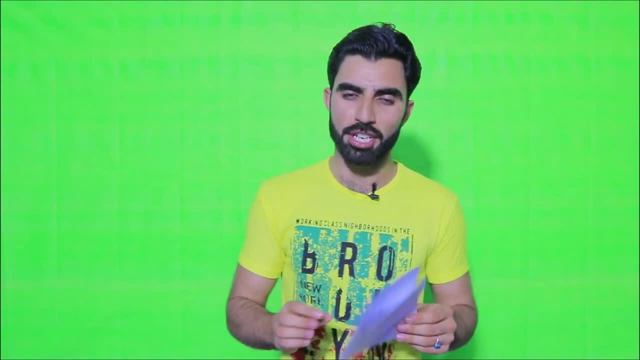 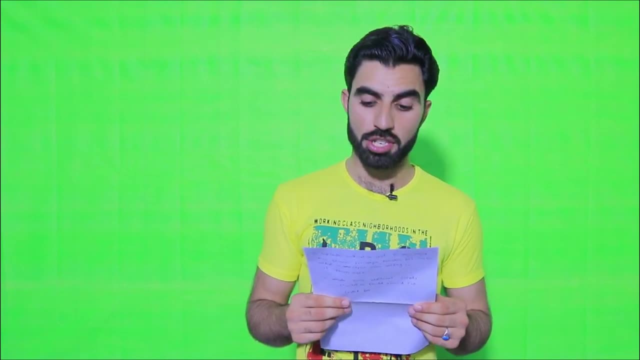 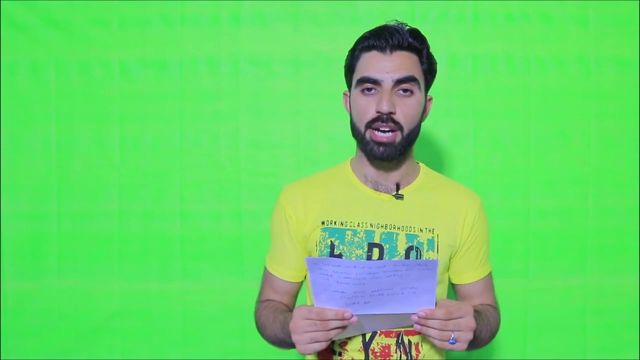 drawing. so let's start, guys, and you should remember if you are studying in seven engineering right. so, guys, as you know, the topic is general notes or general knowledge about steel structure design. so the first one is about, uh, main bars and distribution bars. as you know, we have two types of free bars. 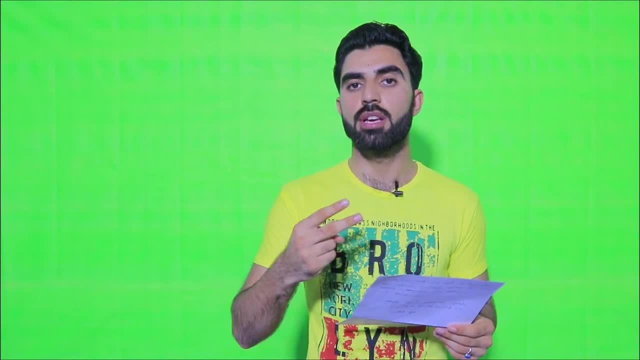 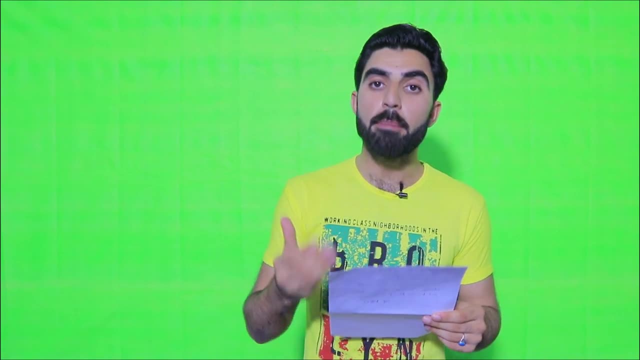 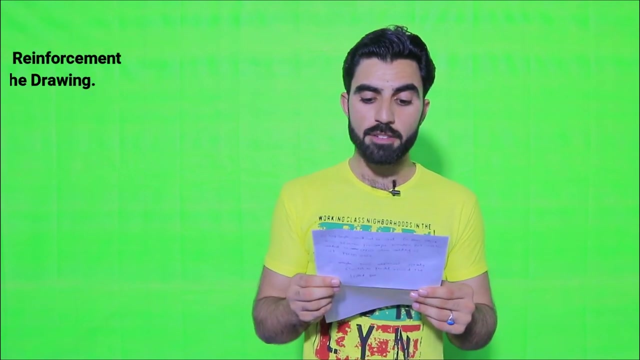 in rcc slip. one is main bar, the second one is distribution bars. so all the positive bottom reinforcement means all the uh, all the main bars in rcc slip, as you know, main bars placed at the bottom in rcc slip. so all the positive bottom reinforcement bars is shown as solid lines in 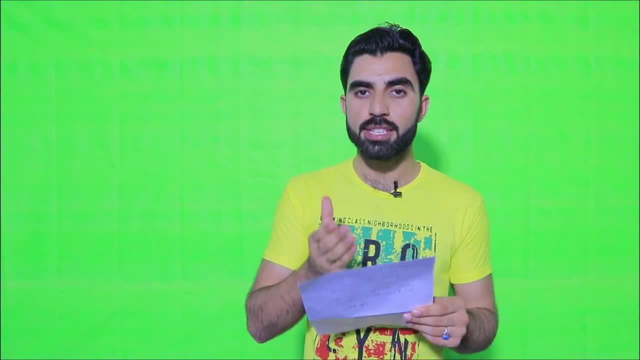 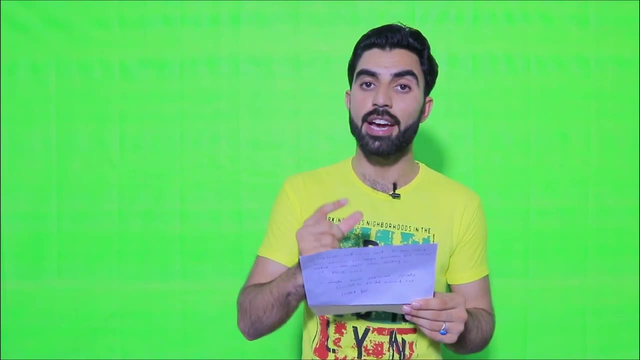 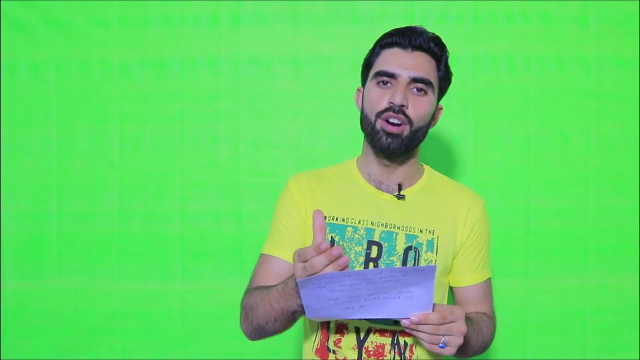 the drawing. so means main bars in rcc, slip, nrcc drawing should be shown as a solid lines, not as a dash or dotted lines or hidden lines, but it should be shown as solid line. so it is useful for as a site engineer, also for if you are working on. 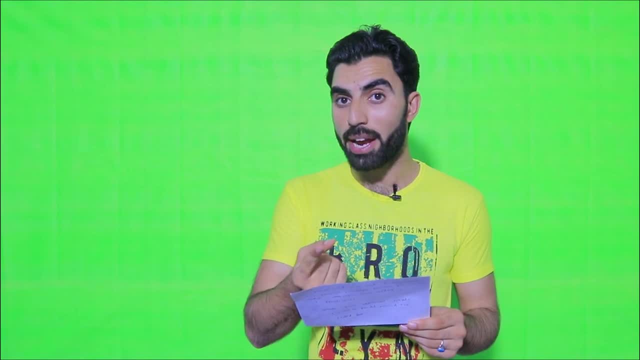 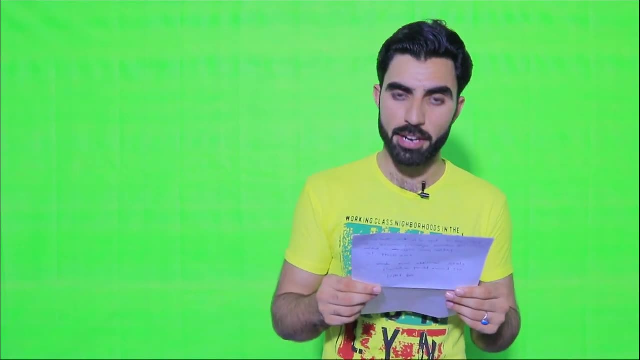 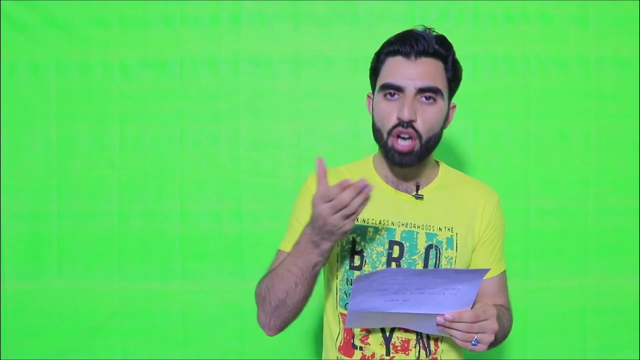 construction site. so you should remember that main bars should be shown as as a solid lines. the second one is about distribution bars. it is also called negative top reinforcement, so all the negative top reinforcement. as you know, our distribution bars are placed in rcc slip at the 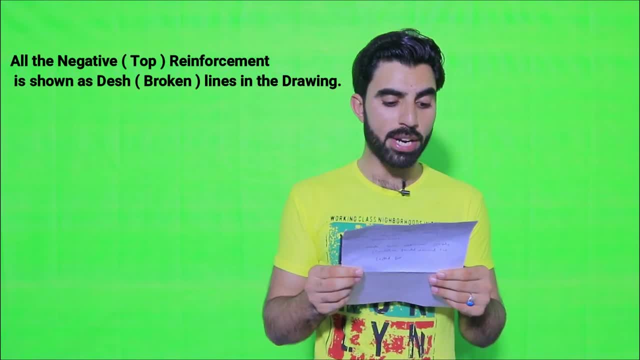 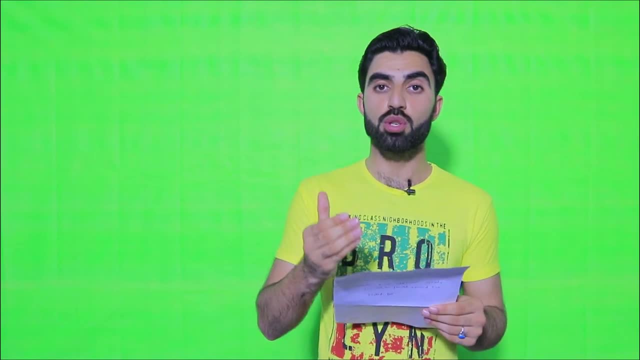 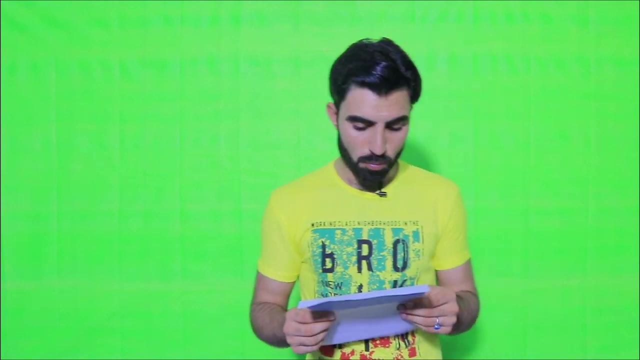 top. so the top reinforcement bars is shown as dash are broken lines in the drawing. so reinforcement- the distribution bars should be shown as broken are dash lines. okay, so this is very useful. these are two points. the third one is lap length for m20 grade concrete. what should be the lapping length? 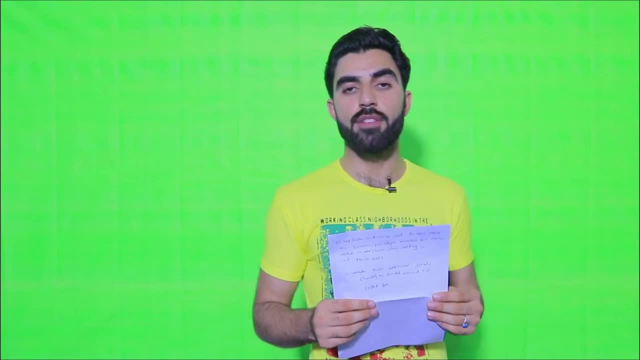 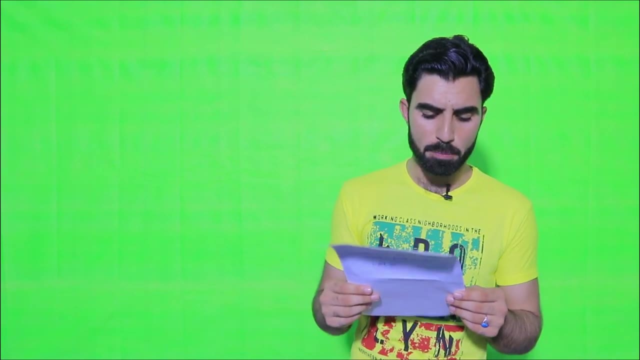 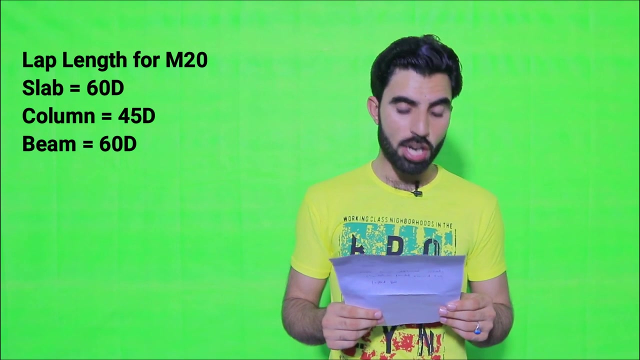 m20 grade concrete. for m20 grade concrete, as you know, the ratio of m20 grade concrete is one ratio: 1.5, ratio 3. so here lapping length is specially for slip column and beam. so, guys, this is from my personal experience and from many research. i got it that the slip lapping length for m20 grade concrete 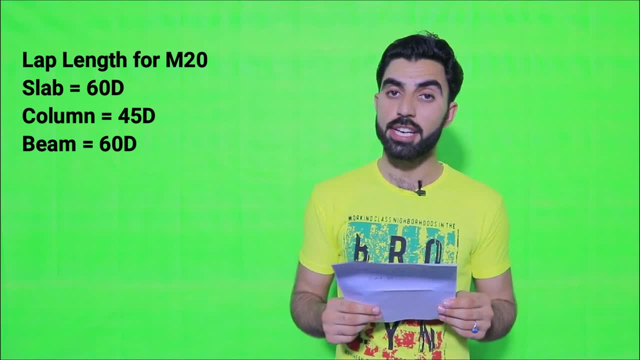 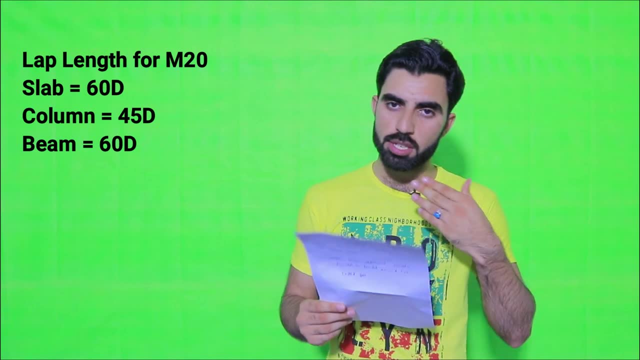 should be with 60d: 60 as a constant and d as a die of steel bar. if that is main bar of our m20 grade concrete, that is distribution bars. okay, so d is die of steel bar. so the slip lap should be with 60d, which is 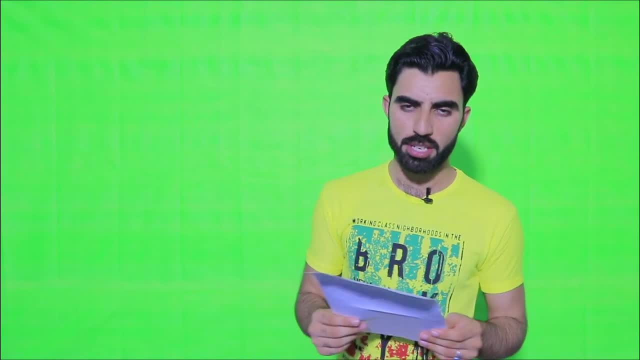 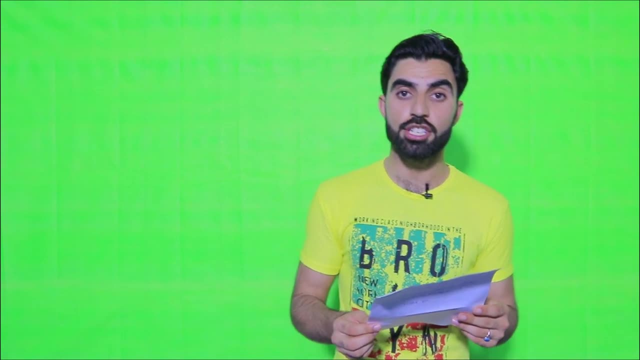 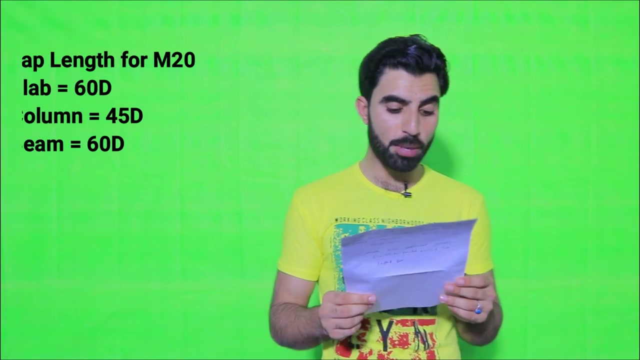 intention. okay, so it should not be maximum 60d. okay, so it's depend on the steel structure design, because it's also depend on the structure load. okay, but 60d is sufficient. the second one is column. what should be the lapping length for the column for m20 grade concrete? so that should be. 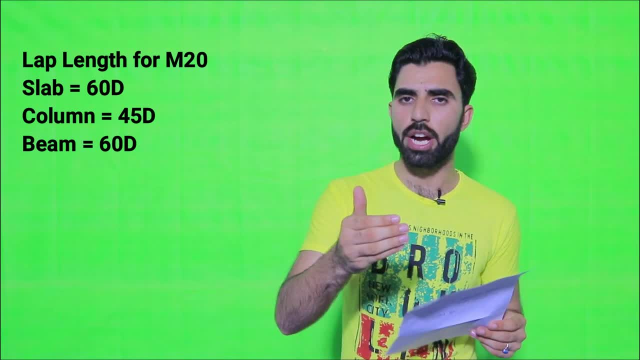 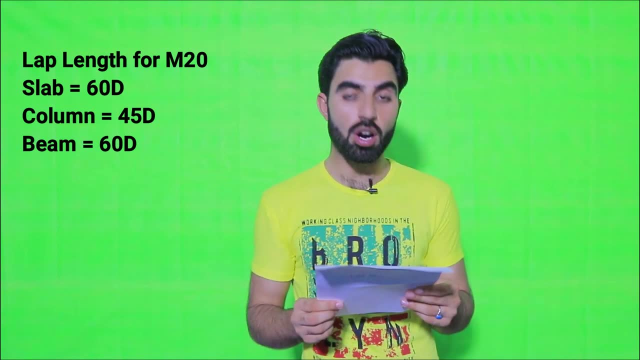 45d or it is depend on your drawing or your structure drawing. okay, but you should show an rcc drawing that the slip is 60d. the column for the column 45d where d is die of steel bar and column is as compression member. okay, so that is. 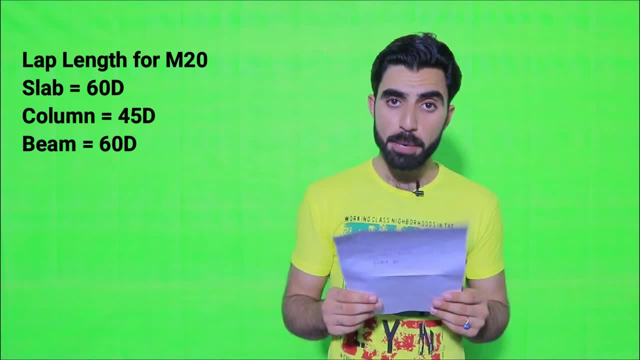 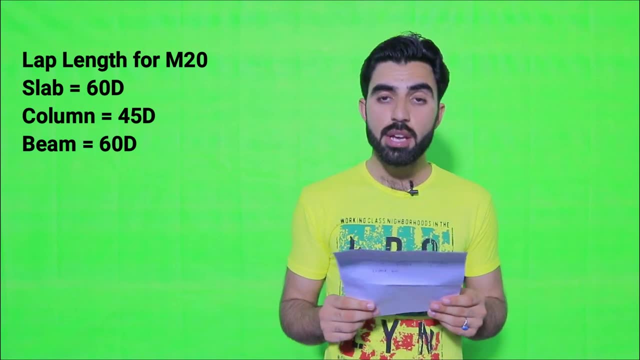 45d. again we have the other one that is beam. so the beam is tension member, so it is also 60d. so slip and beam. for that the formula of lapping length should be 60d, and for the column 45d is sufficient. okay, guys, the fourth point is concrete. 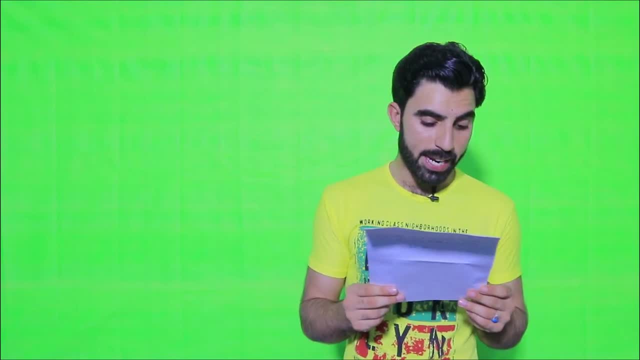 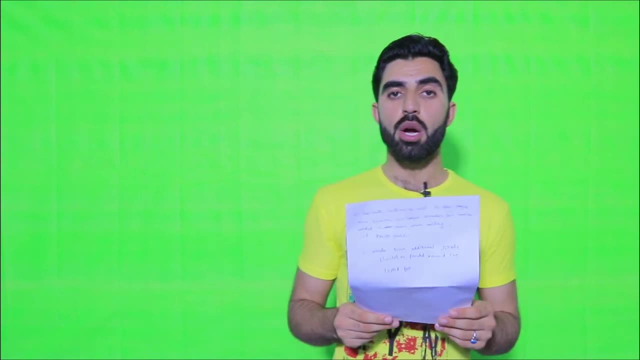 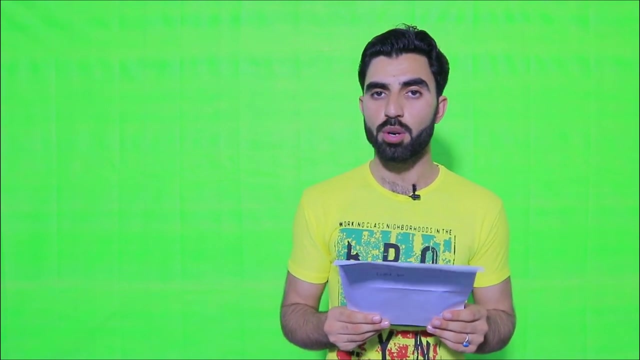 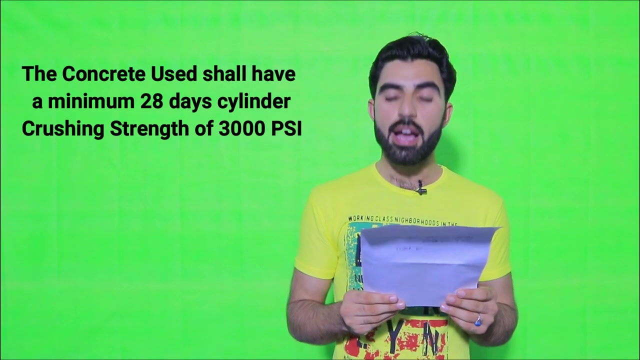 used shall have minimum 28 days cylinder crushing strength of 3000 psi per square inch. so, as you know, we can get the 3000 psi. the concrete mix should be m20 grade, okay, so when you want to grade m20 grade concrete, full strength. so the concrete used shall have a minimum 28 days cylinder crushing. 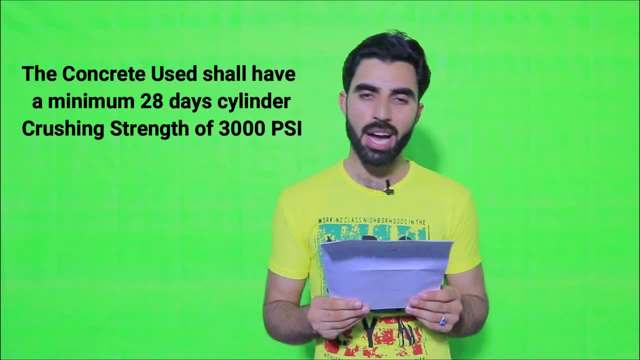 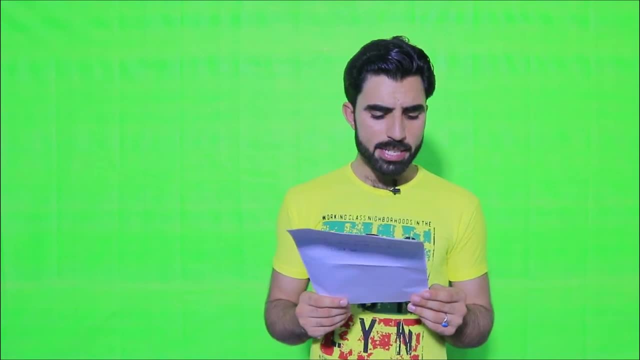 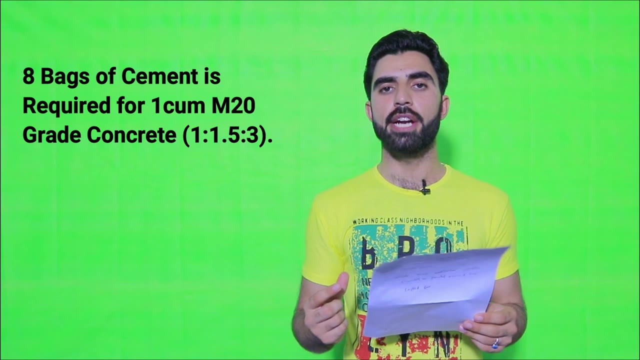 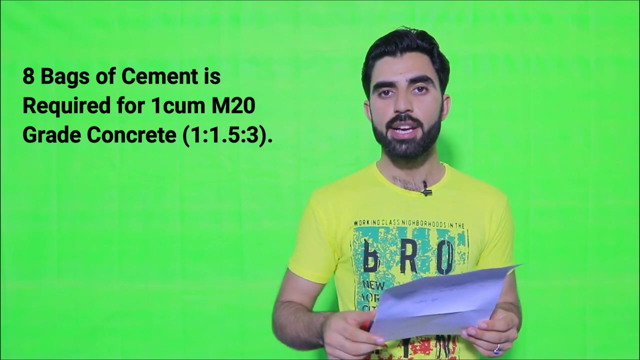 strength of 3000 psi. right, this is the other useful point and you should write in our cca drawing: okay, guys. the fifth one is eight bags cement is required. if someone asks from you that how many bags of cement is required for one cubic meter concrete in m20, in m20, okay, m20, one ratio. 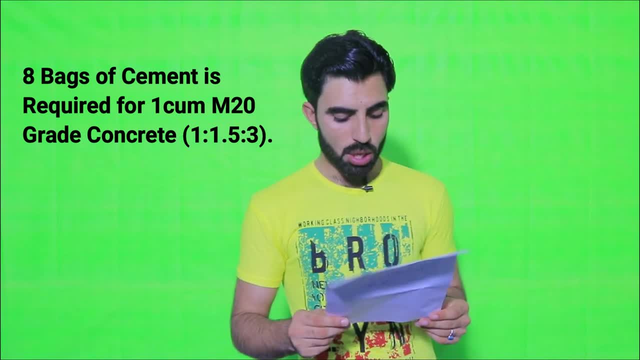 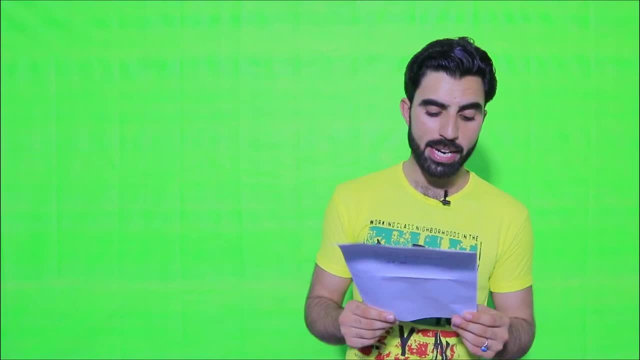 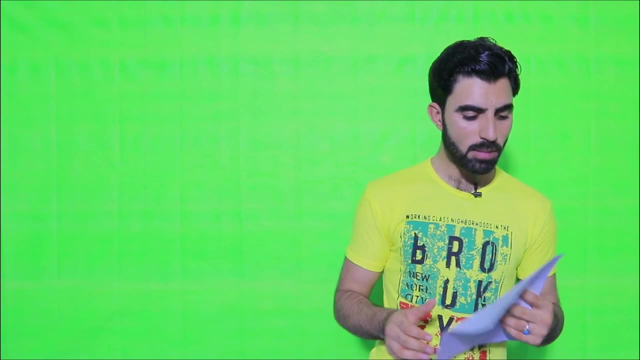 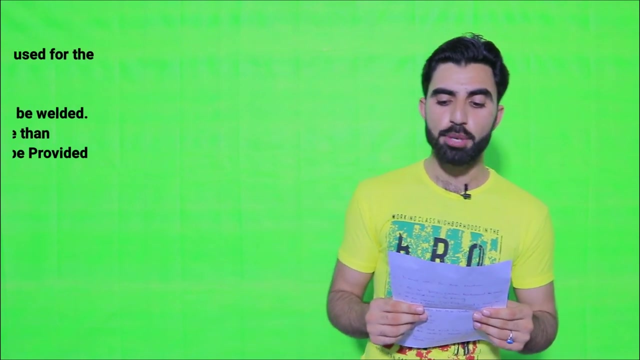 one ratio, 1.5, ratio 3. so for m20 grade concrete, for one cubic meter, we required an m20 m20, we required eight numbers of bags, and each bag weight should be 50 kg. right guys? the last one is very useful. this is the sixth point. lip length shall not be used for the bar. 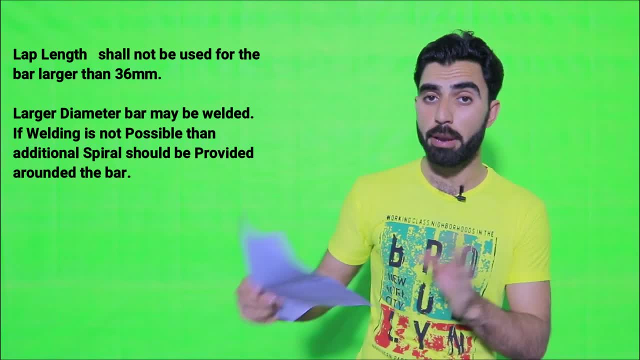 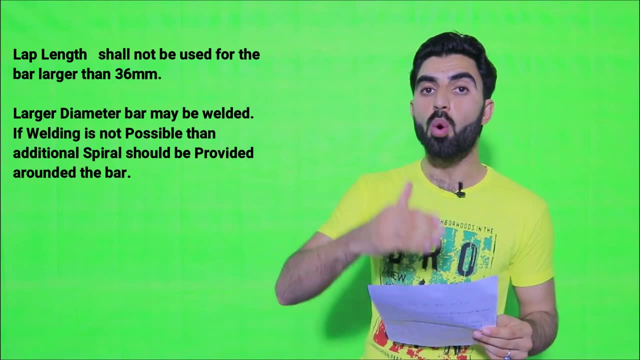 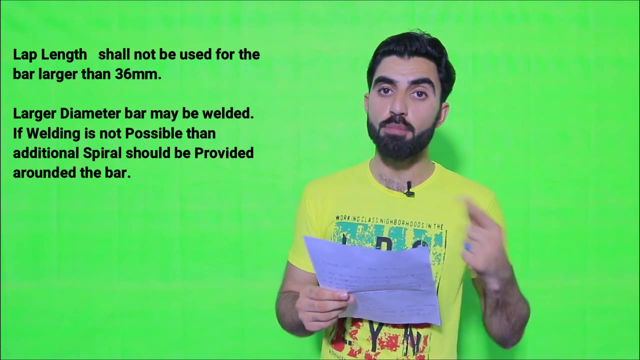 larger than 36 millimeter. as i told you in many videos that the lapping length should not be allowed if the die of steel is more than 36 millimeter. what we should do, okay, so for larger diameter, it means more than 36 millimeter bar diameter.